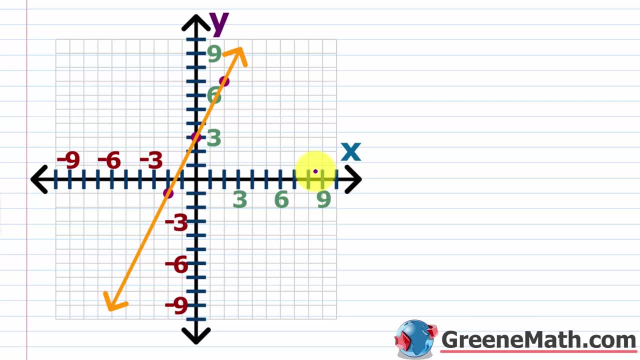 So for this guy right here, this line, let's just get the equation going. We know the y-intercept occurs where- Let me make that better. The y-intercept occurs where It's going to be right here, So it's 0,3.. So, 0,3.. And the slope is what? If I started at this point right here and I wanted, 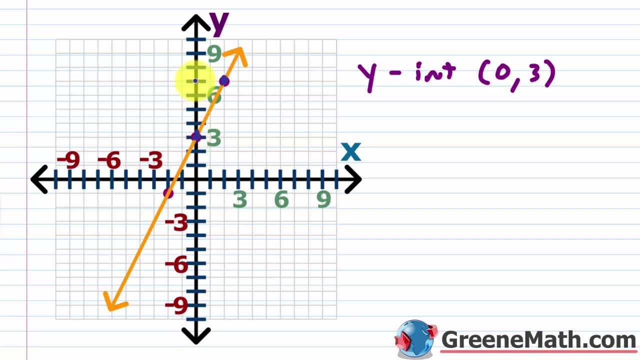 to go to this point, I would rise 1, 2,, 3,, 4, and I would run to the right: 1, 2.. So m my slope again is rise over run, And in this case it's going to be 4 over 2,, which is 2, right And. 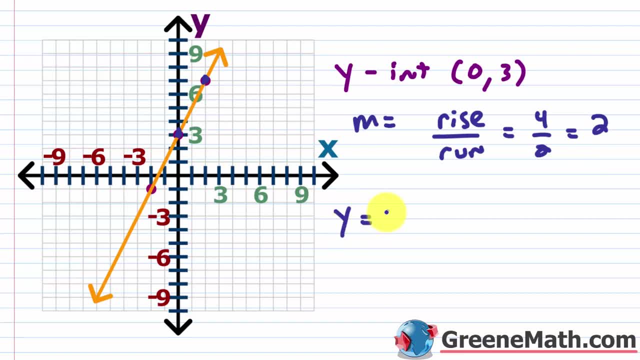 specifically here, it's positive 2.. So we can say the equation is: y equals 2, my slope times x plus 3, my y-intercept. Or if you want to use function notation, you could say: f of x equals 2x plus 3.. 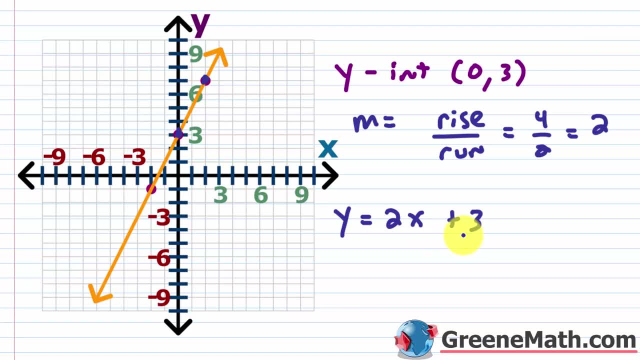 That's up to you, But the main takeaway here is that with a positively sloped line, essentially as x increases or as we move to the right, y also increases, And with a line, because the slope is always the same, it's always increasing. 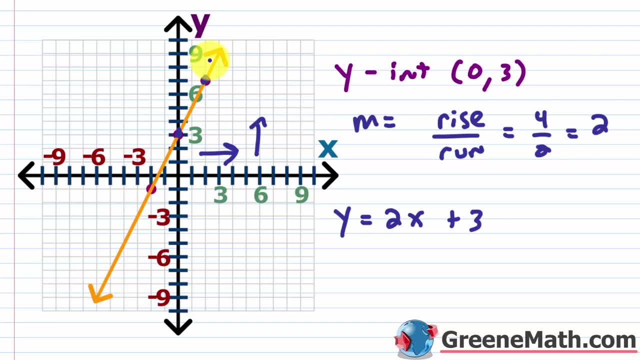 it's always constant or it's always decreasing. It's one of those three things, unless you have a vertical line where the slope is undefined, But in this particular case again, because we have a positively sloped line as x increases as we move to the right on the x-axis. 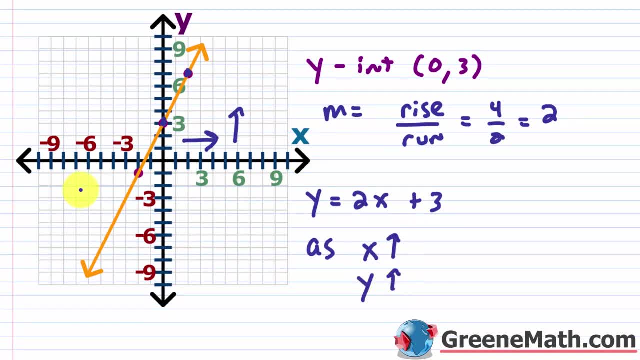 y is going to increase. So we can say that this function- this y equals 2x plus 3, or f of x equals 2x plus 3, is increasing kind of over its whole domain. okay, So the way we want. 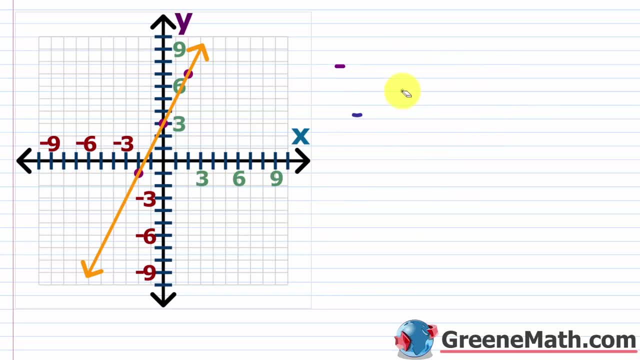 to write this. let me just erase all this. When you get in this section, they're going to ask you for the intervals where it's increasing, decreasing or constant. So we're going to say increasing And I'll say on the interval: Well, for here it's going to be from negative, infinity to positive. 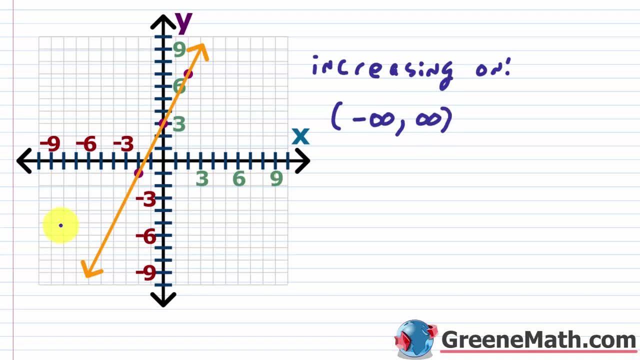 infinity again across its entire domain, right? So if I go all the way to the left, as far as I can go, this arrow here that indicates it continues forever in the negative direction. as I go to the right, as far as I can go, it's always increasing. okay, So, from negative infinity. 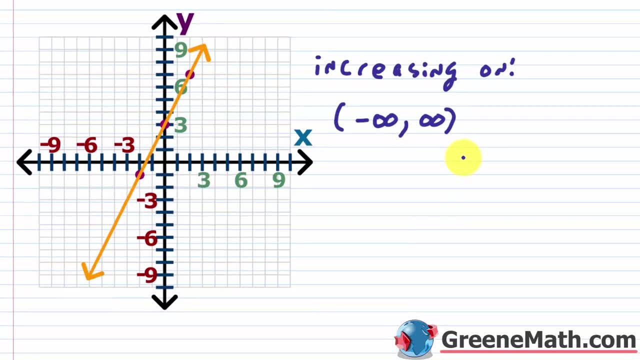 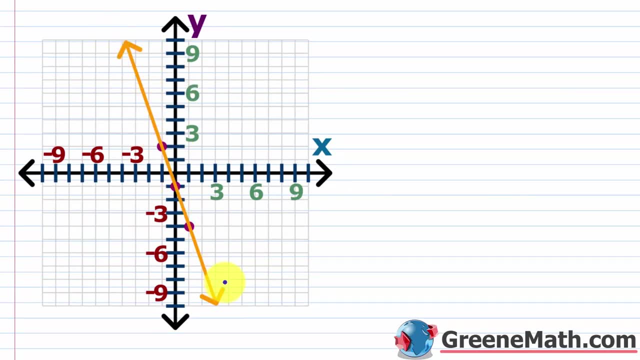 to positive infinity. it's never decreasing and it's never going to be constant. All right, we also have negatively sloped lines, And for this guy the reverse is going to be true. So for its entire domain, this function is going to be decreasing As x values increase or we move. 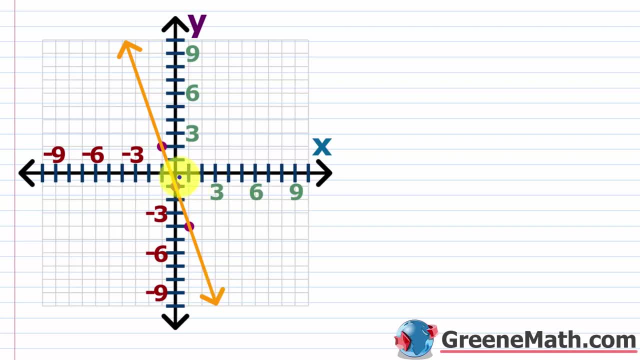 to the right, y is going to decrease. So let's kind of do this formally. So this guy right here: the y-intercept is going to occur at 0, negative 1. And the slope m is going to be 1.. 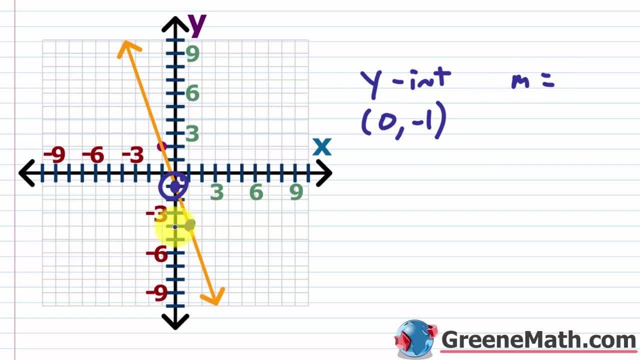 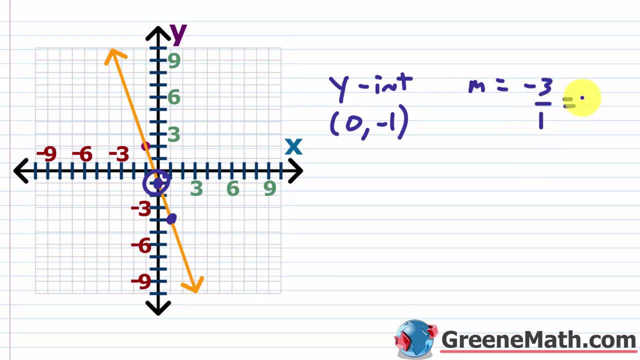 If I want to go from this point to this point, I've got to fall 1,, 2,, 3, run to the right 1.. So that's negative 3 for the rise and it's a positive 1 for the run. So this is just negative. 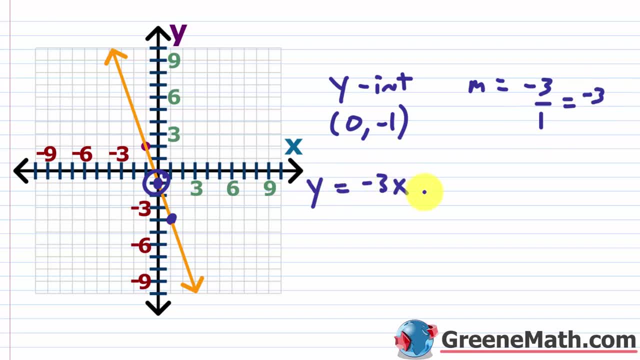 3.. So I would say y equals negative 3x and then minus 1.. Or again you could say f of x equals negative 3x minus 1, if you want to use your function notation. But the main takeaway: 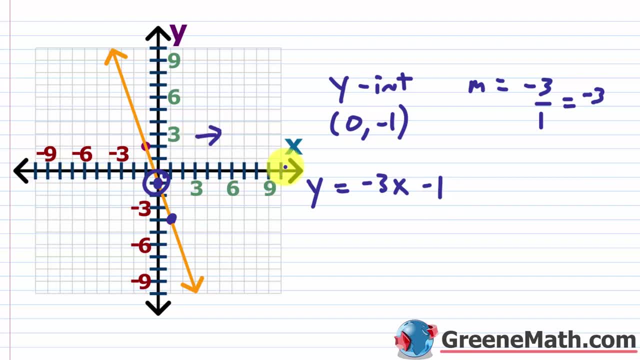 again, as x increases as we move to the right on the x-axis, y is always decreasing, And this is from negative infinity out to positive infinity. So I'll say decreasing again on this interval from negative infinity to positive infinity. Again, it's not increasing. 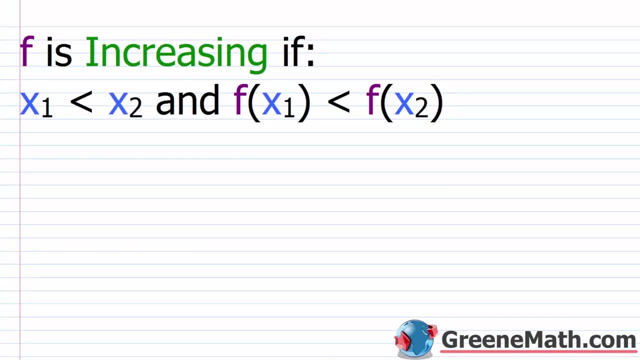 anywhere and it's not constant anywhere. All right, so just to recap, when working with lines, the process is really easy. In fact, you're never going to get a line in the section. I'm just for the purposes of getting our thought processes going. But it's easy because the slope is always. 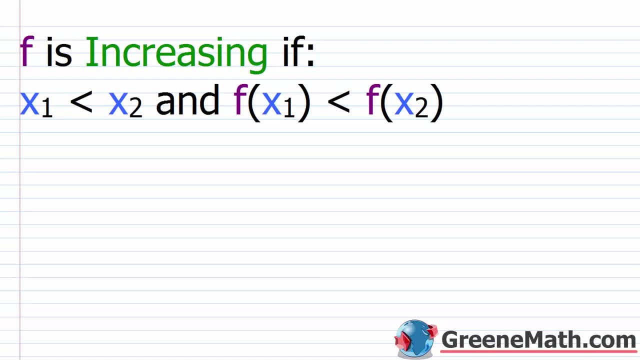 the same. okay. So when a line has a positive slope, it increases across its entire domain, Again from negative infinity to positive infinity, And when a line has a negative slope, it decreases across its entire domain And then, with a horizontal line, it's constant across its. 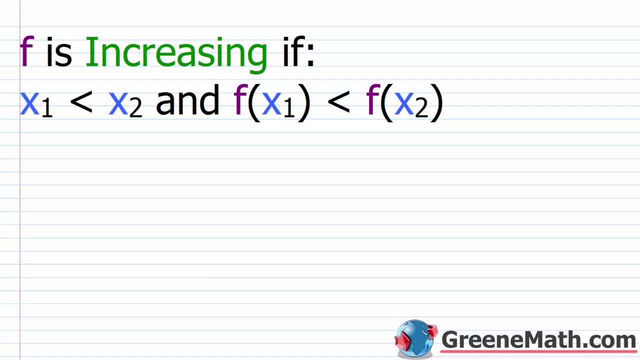 entire domain. Now, in most cases, and I would say pretty much in every case, you're going to be dealing with something that's not as simple as a line, So sometimes our graph is going to make all these weird twists and turns, And so over the span of time we're going to be dealing with 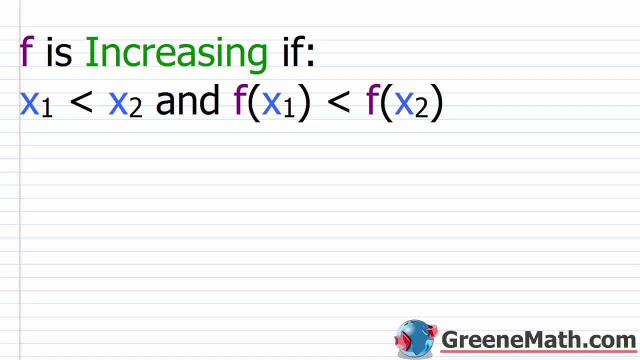 something called the increasing, decreasing and constant, And in the process it's going to change as we go on. So if you look at the line, you may have several changes between increasing, decreasing and constant. Again, when you get to calculus you'll be able to use the derivative. 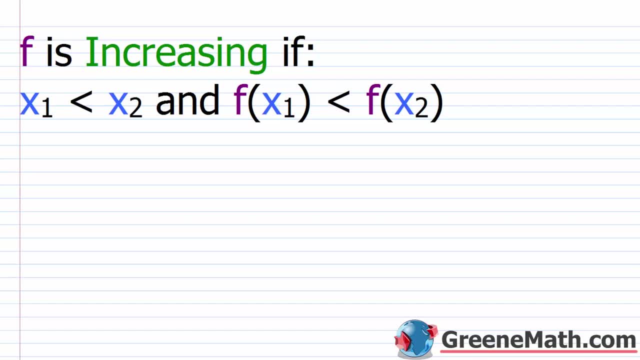 to kind of find the increasing intervals, the decreasing intervals and the constant intervals. But for right now that's a bit beyond us. So let's just observe this kind of general definition and then we'll move on and look at some kind of graphs. So f our function is increasing. 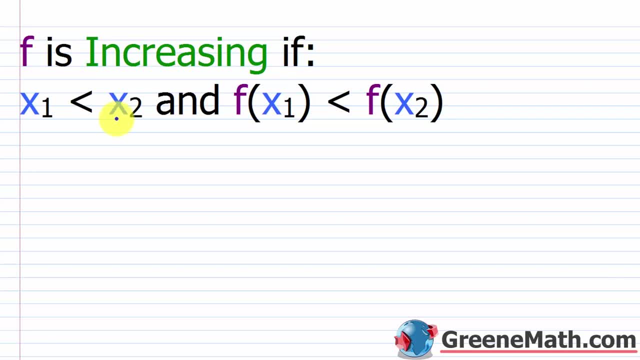 if, across this given interval that we're looking at for any two x values- let's call them x sub 1- we could say that x sub 1 is less than x sub 2, and f of x sub 1 is less than f of x sub 2.. 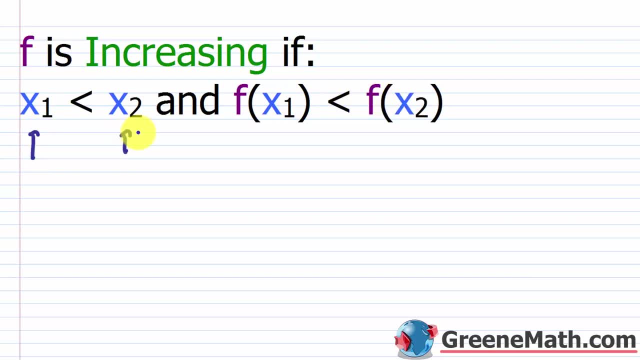 So what this means is that this x value is smaller than this x value, So this x value is to the left of this one. okay, Then plugging in this x sub 1, this smaller x value for the function and kind of getting the output results in a smaller value than using the larger x value as an input right. 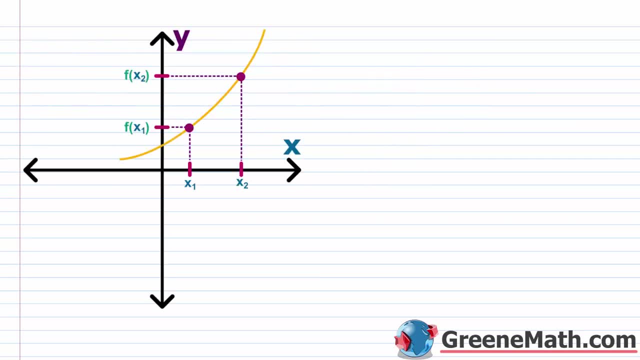 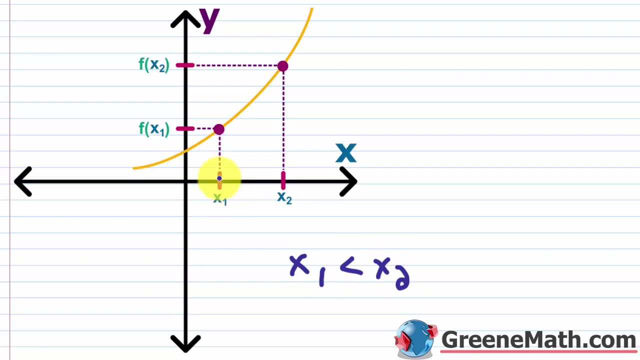 The output there is larger. So to see this graphically, we see again that x sub 1 is to the left of x sub 2.. So we know that means that x sub 1 is less than x sub 2.. And we see that. if I kind. 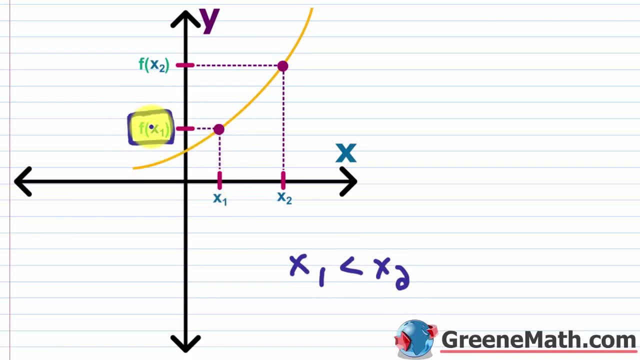 of go up here the f of x sub 1 or the y value associated with plugging in an x sub 1 for each occurrence of x in that function is smaller than f of x sub 2, right The y value associated with. 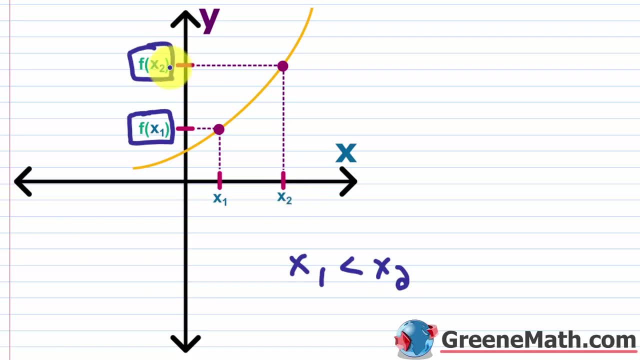 plugging in the larger x or the x sub 2 for each occurrence of x in that function. So we can say that this function is smaller than f of x sub 2,. right, The y value associated with plugging in the larger x or the x sub 2 for each occurrence of x in that function. So we can say that this function. 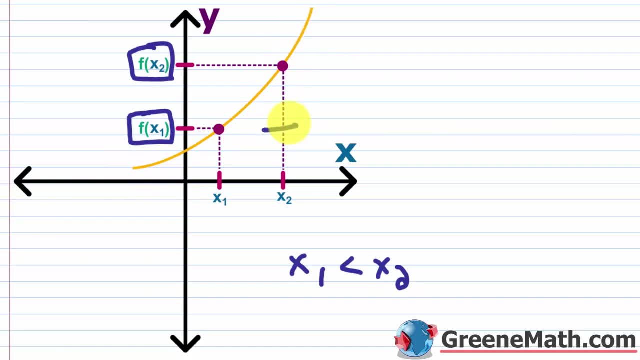 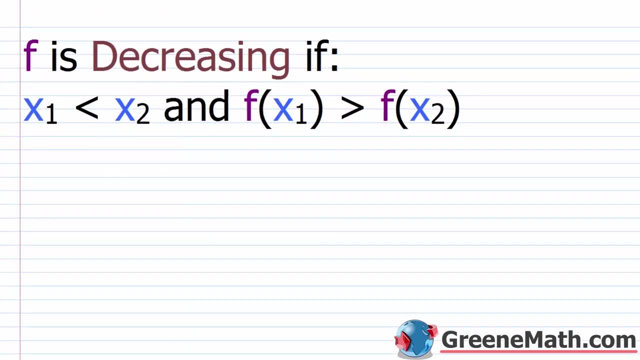 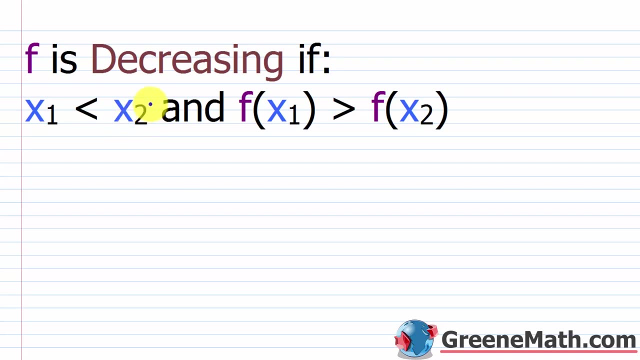 is increasing right As we go from left to right, the function is increasing over that interval. if the y values are increasing over that interval- Right now also, you'll see f is decreasing, if kind of the reverse is true. So we have x sub 1 is less than x sub 2.. So this part's still the same. 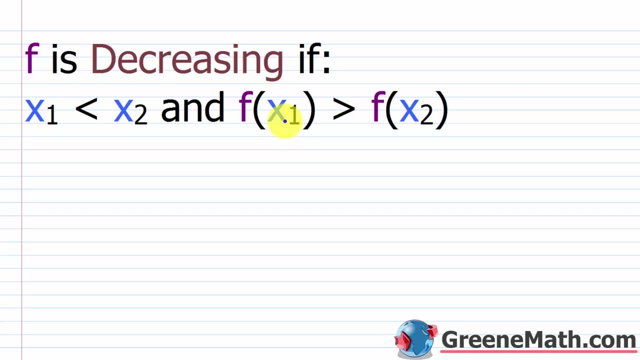 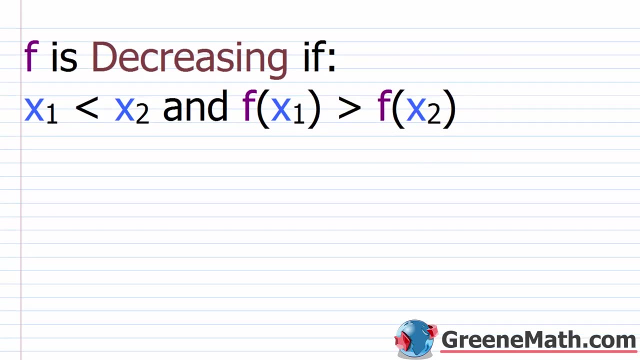 x sub 1 is still smaller. But now f of x sub 1 is greater than f of x sub 2.. So plugging in the larger x value right now we're getting a smaller output here. So when we look at this again, 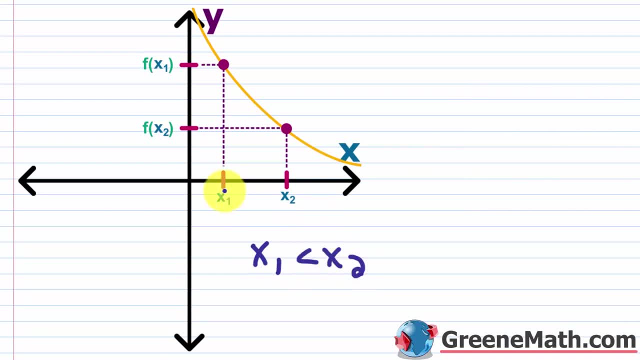 x sub 1 is less than x sub 2.. We see that f of x sub 1 is higher than f of x sub 2.. So this graph is falling as we move to the right, So it's decreasing over this interval. Now, lastly, we might see where 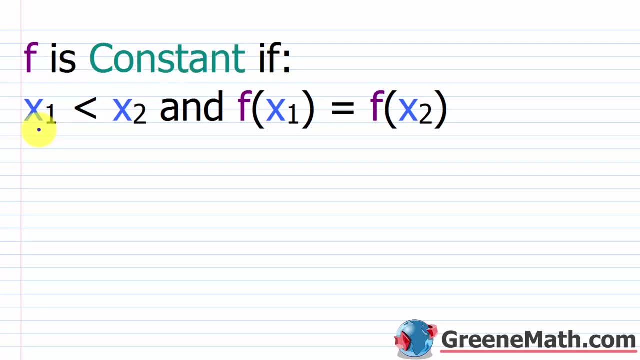 it's constant. So we can say f, our function is constant if x sub 1 is less than x sub 2 and f of x sub 1 is equal to f of x sub 2.. So we can see that f of x sub 1 is higher than f of x sub 2.. So this: 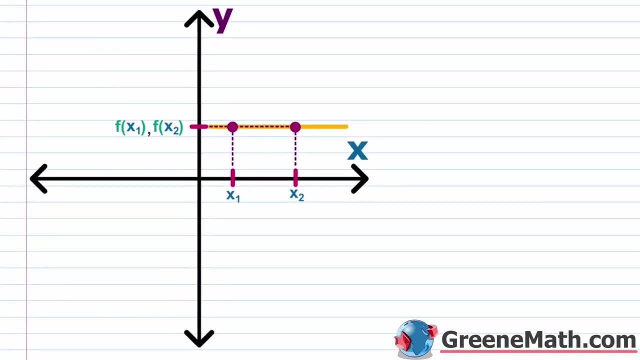 is f of x sub 2.. So we all know what a horizontal line looks like And essentially, over this interval you have any given x sub 1 and x sub 2.. x sub 1, again, is less than x sub 2.. And the 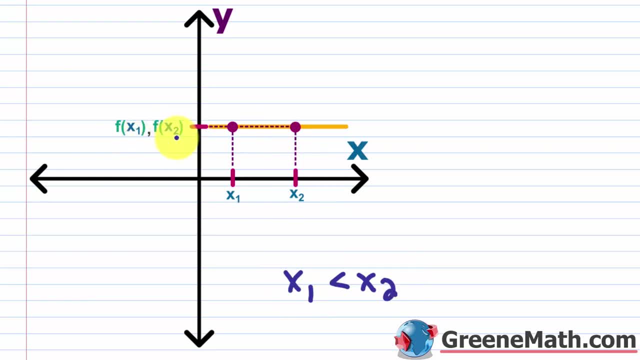 y values here are the same, So f of x sub 1 is the same as f of x sub 2.. This generates a horizontal line, So here the function is just constant. All right, let's take a look at the first example. 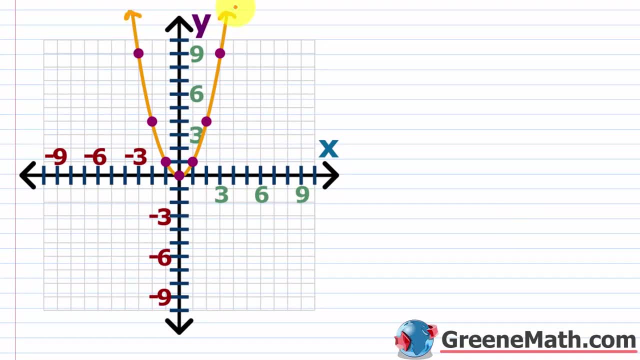 here. So I'm just going to put some arrows on this And I'm going to say that this is y equals x squared. We've already seen this graph before in a previous lesson, So with this guy again, I want to determine the intervals where it's increasing. 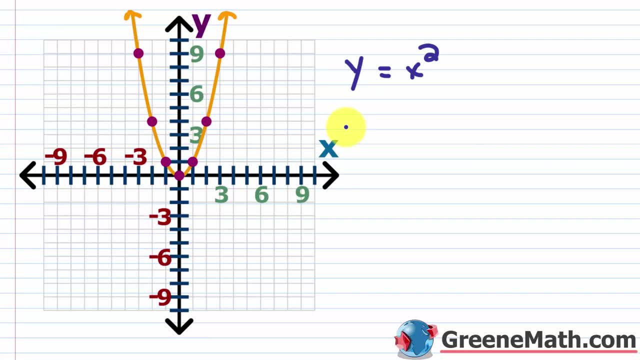 decreasing or constant. So what I'm going to do is I'm going to start from kind of out here all the way to the left, from negative infinity, to kind of going this way. what happens? Well, if I look at my y values, if I kind of think about it, I'm decreasing right As I'm going. 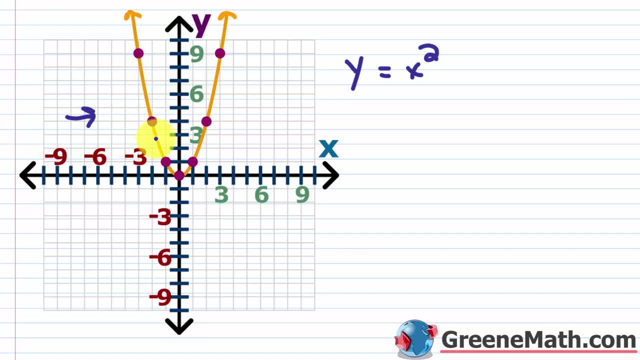 to the right. I'm decreasing, decreasing, decreasing, decreasing, decreasing, until I get to zero, okay, And then, after zero, then I'm increasing, decreasing, decreasing, decreasing, increasing, increasing, increasing, increasing. A lot of people will draw like a stick figure. 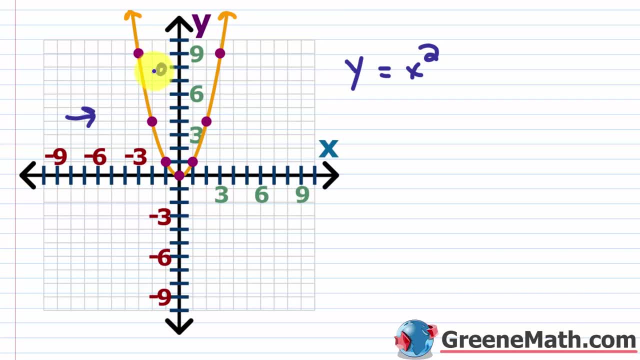 or a car or something like that to kind of illustrate. I'm not a good drawer, but I'll try my best. So my stick figure there would be walking downhill until he gets to zero, And then after zero he'd kind of be walking uphill. So let me do that So you can see. 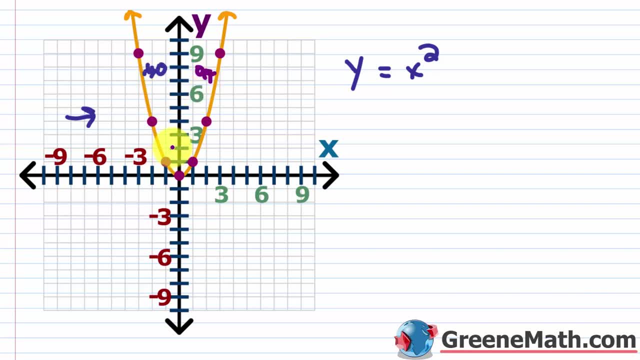 that there. It's not a good drawing, but you get the idea. Another way you can think about this is if I kind of think about an x value of negative three corresponds to a y value of positive nine. If I increase the x value by one, if I go to negative two. well now 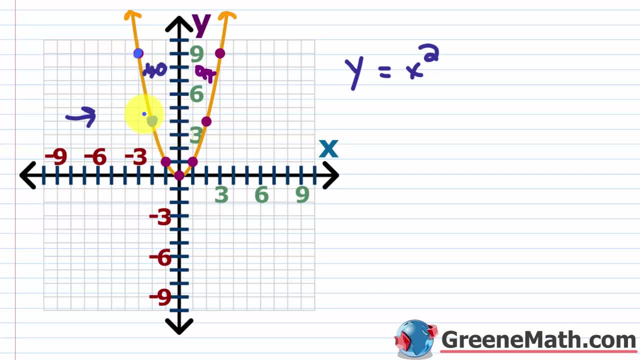 my y value is positive four. So increasing x resulted in me decreasing y. So again, that's how I know- I'm decreasing again until I get to zero, And then I start increasing right. If I look at an x value of two, I get a y value of four. If I look at an x value of 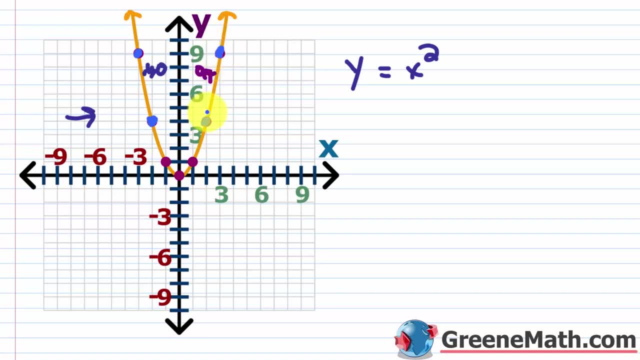 three, I now get a y value of nine. Okay, So that's another way you can kind of think about this. So we can say that in terms of the, the intervals, we are decreasing on the interval from a negative infinity up to, but not including, 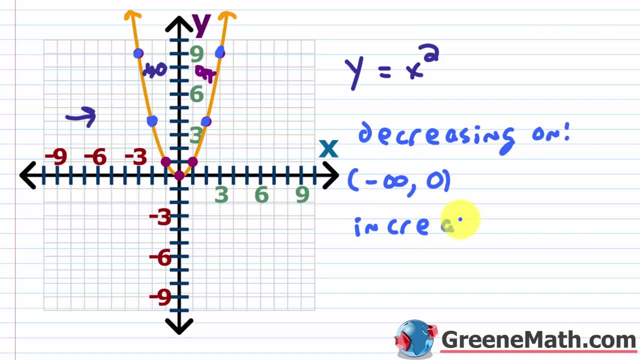 zero and then we're increasing. we are increasing on the interval, again not including zero, out to positive infinity. So you might be asking: why didn't I include zero? and you might also be arguing saying that your book includes zero. So these are both valid points. 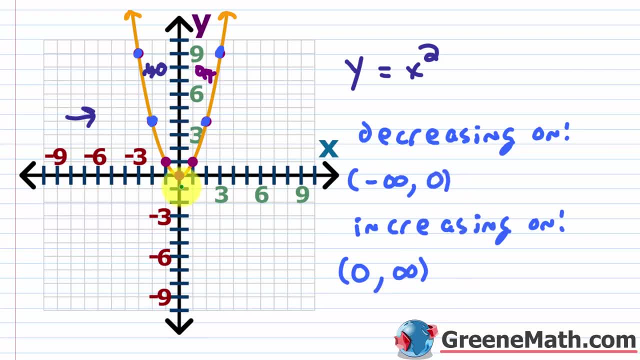 So the first thing is that I didn't include zero, because if you think about what happens to this function when you're at zero, you're not increasing and you're not decreasing, In fact, the slope there. if you took the derivative and you looked at it specifically, where x? 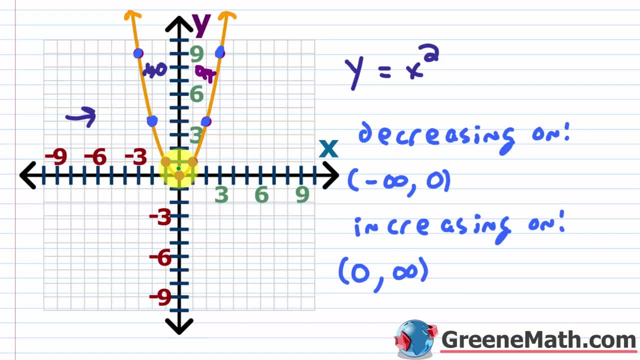 was zero, you'd find that the slope is zero, So it's not positive, it's not negative, it's zero. So that means it's not increasing and it's not decreasing. so that's why I didn't include it. I just used the open notation so that it's excluded. 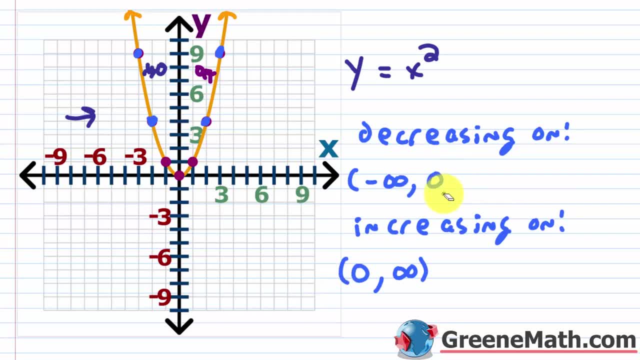 The second point is: your book might show this, Your book might do this. Now, is this wrong? The answer to that question is: I would go with whatever your teacher tells you to do, because ultimately, they're grading your test. Most books- I would say the majority of them- and most teachers are going to want you to. 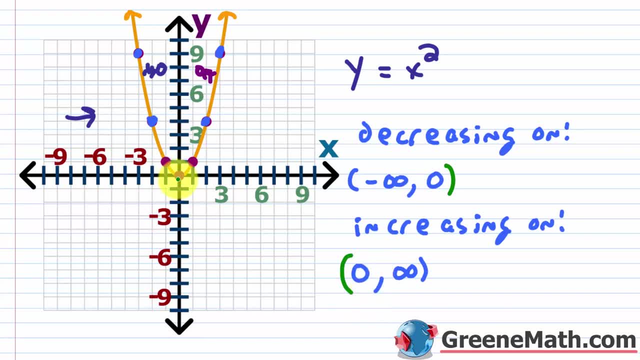 use this notation here for the point that I just made. At zero, it's not increasing and it's not decreasing, so it's not included in either of these intervals. Okay, So this is this kind of bracket notation: Follow your book, follow your teacher, go with what they tell you. 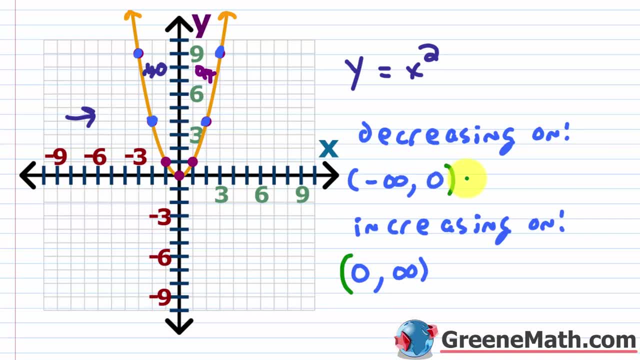 Now, the other thing that you want to consider here is that when we list the intervals, it's in terms of x values, We're not listing ordered pairs and we're not listing y values. so don't make that mistake. I am considering what is happening to the function, what is happening to, kind of the 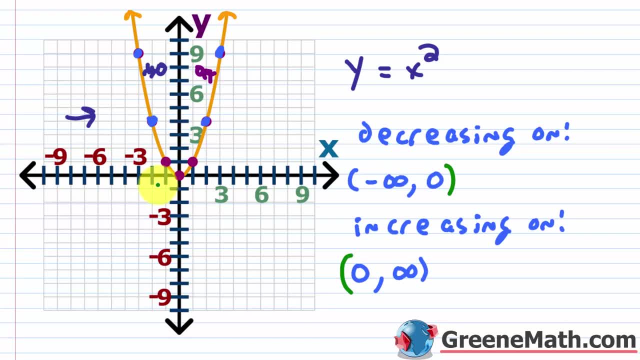 y values. as I kind of look at these intervals on the x axis, So from the interval negative infinity up to, but not including, zero, the function is decreasing, So the y values are decreasing. Then when x is larger than zero we can say the y values are increasing again. so the function 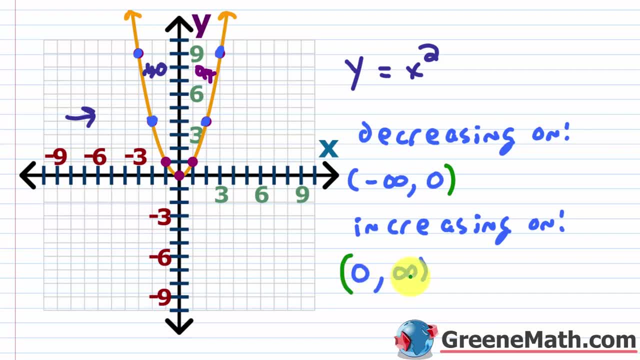 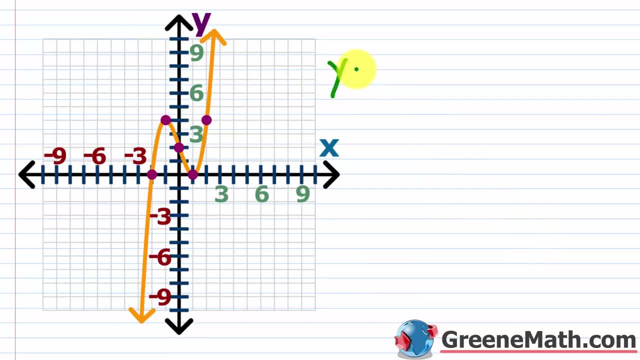 is increasing over that interval from zero out to positive infinity. So it's always in terms of the x values. That's what you're writing. All right, Let's take a look at another one. So this is the graph of y equals. we're going to have x cubed minus. we're going to have 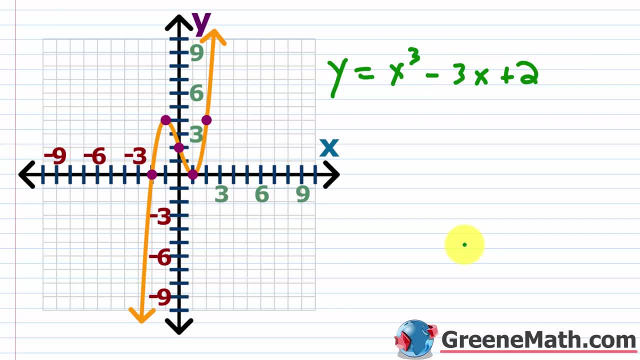 three x and then plus two. For right now we just want to observe from the graph where it's increasing, where it's decreasing and where it may be constant. Well, again, if I kind of think about things coming from negative infinity going to positive, 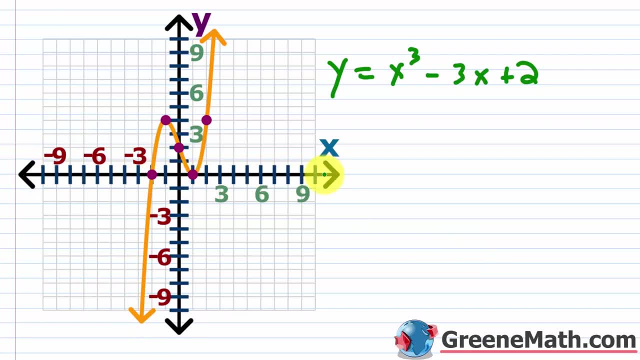 infinity. So again I'm thinking about what's happening as I move across the x axis, as I go to the right. So, starting from negative infinity, going up to this kind of negative one on the x axis, I'm increasing Right, So I can again draw my little stick figure. 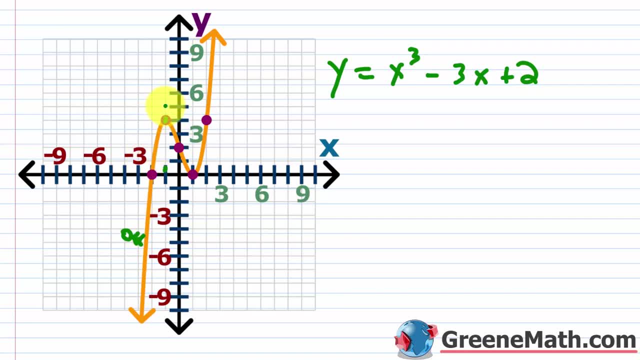 This guy would be walking uphill the whole time. When he gets to an x value of negative one, he would kind of change and then, right here, he would be walking Downhill. So he'd be walking downhill until he got to an x value of positive one. 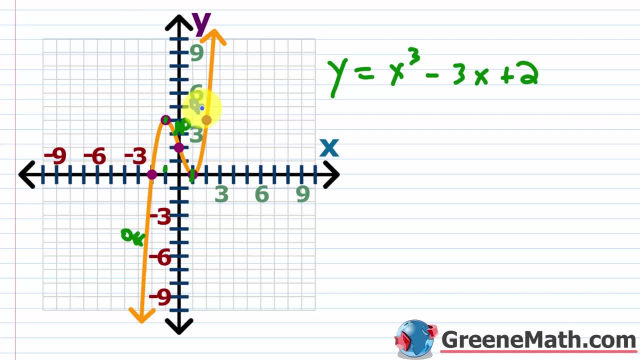 And then he would be walking uphill again from positive one, that x value, out to positive infinity. Okay, So if you think about it this way, for the increasing intervals, so it would be increasing on, okay, the intervals. one interval would be from negative infinity up to, but not including, 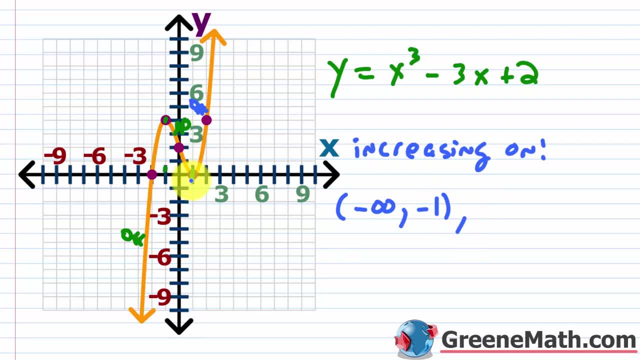 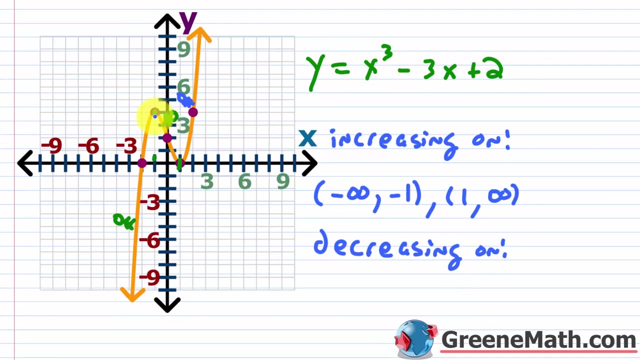 negative one. Another interval would be from positive one and then out to positive infinity. Now let's talk about the decreasing. So we'll say: is decreasing on what interval? So that's going to be from negative one to positive one. Again, I'm not going to include either one of those. 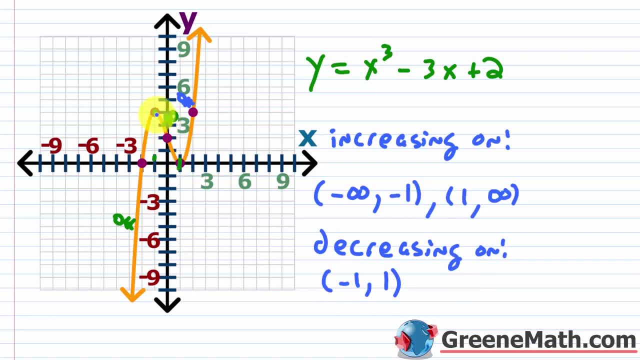 So at negative one and positive one, you kind of have these turning points here and the slope here, the derivative of the function. When x is negative one and when x is positive one, it's going to be zero. So I'm not going to say it's increasing and I'm not going to say it's decreasing. 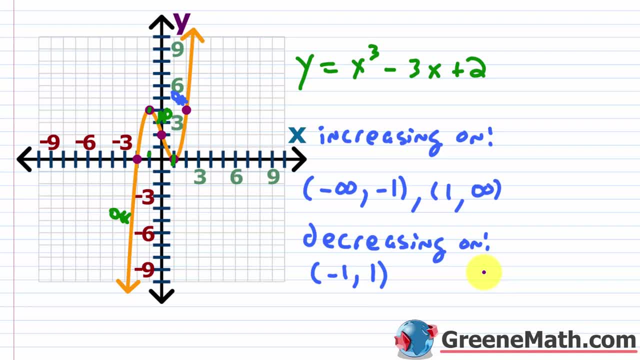 Okay, Before we move on to the next problem, I want to talk about another common source of confusion. So if your book specifically asks you for the intervals where this function's increasing, decreasing or constant, you don't want to put a union symbol in here. 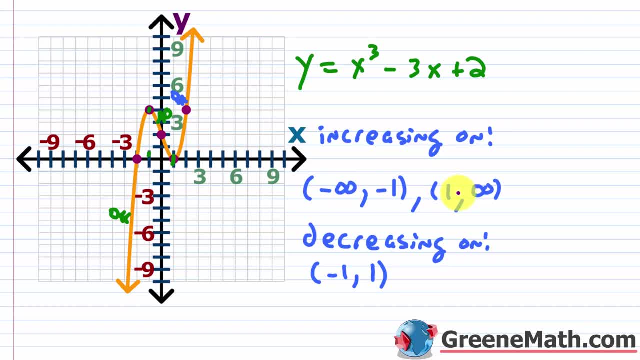 Okay, You see that a lot. So sometimes you have more than one interval involved in one of your answers, So you'll see students go: okay, it's this, It's this guy, And then union with this guy. That's not correct. 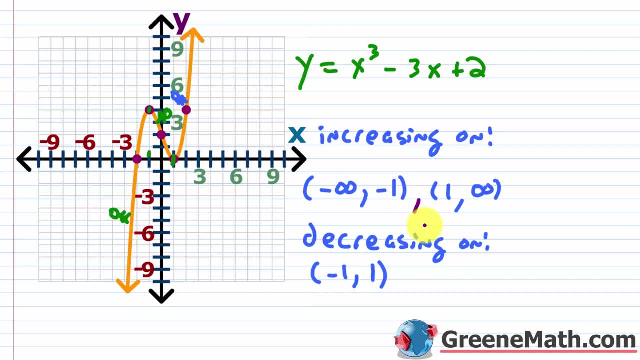 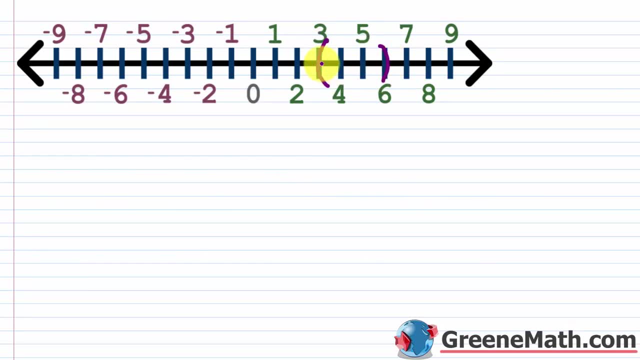 So if I'm asking you for an interval, what am I asking you for? Let's go to a number line real quick and think about this. Let's add an interval from three to six, with three and six not included. So that's this interval here. 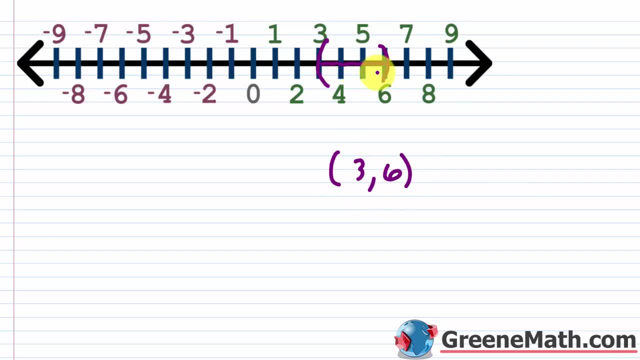 Essentially it's a set of numbers, that's kind of between two numbers, where the endpoints could be included or not included. You can't have a gap right, So you can't say: well, I have another interval from negative five to negative one. 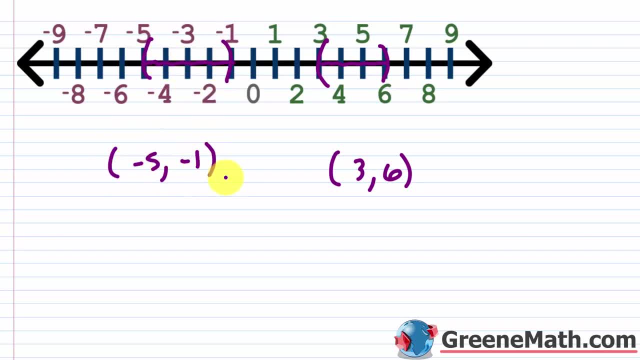 And that's not included. Okay, And let's say, I have this guy right here. I can't just use a union symbol and say, okay, this is now one long kind of interval. Okay, That doesn't make sense. This is a set that contains the union of those two intervals. 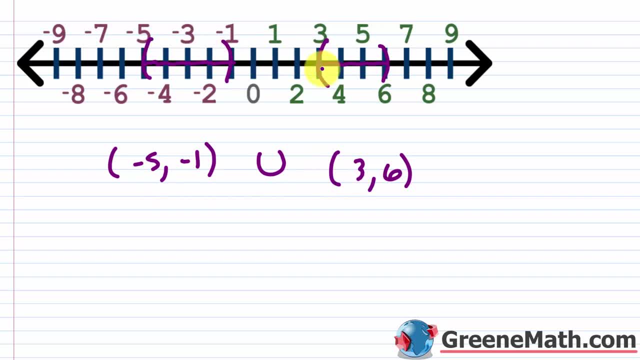 Okay, But it's not one long interval. That wouldn't make any sense. Okay, You can't have a gap like that. So if they're asking you for the intervals- okay, intervals plural- then just put a comma between them or use the word and okay. this is a common trap question. 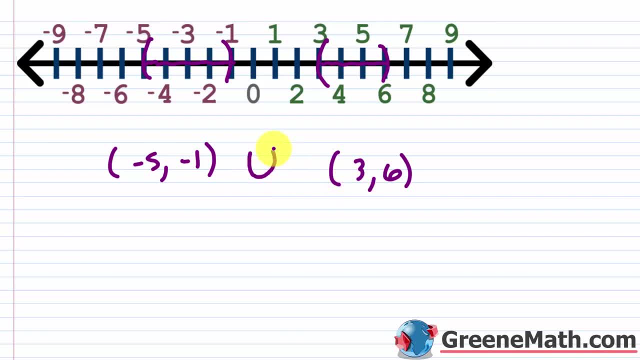 Because they might give you a multiple choice and they might put a union symbol in between the two and they might give you a choice like this and you might be scratching your head and say, okay, well, I've used this a lot. 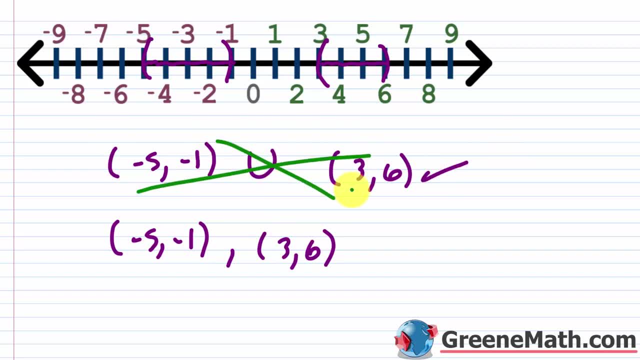 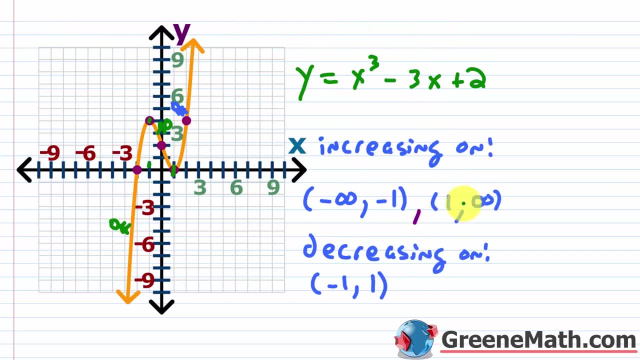 So you might check this one as correct. but what happens is this one would be wrong. Okay, Because they asked you for the intervals, Okay. So if we go back, we want to list it like this, or just put the word and kind of in: 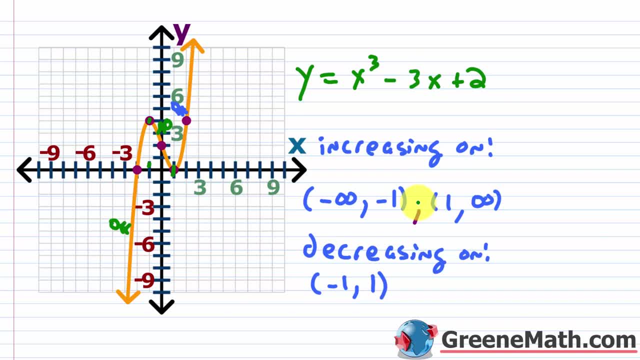 between them If the question is asked differently. okay, this is the thing that gets confusing. Then you might be able to use your union symbol. If we're just talking about where's the function increasing and there's no mention of give the intervals, 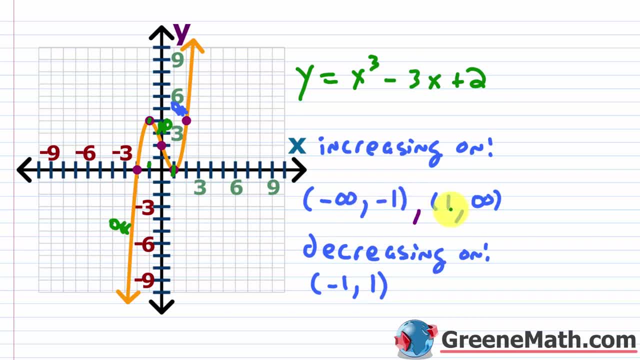 Well then you could give it with that kind of union statement, because you're just looking for the set, that kind of satisfies, that answer, And that set would contain these two intervals, and you could join those with a union symbol. That would be fine. 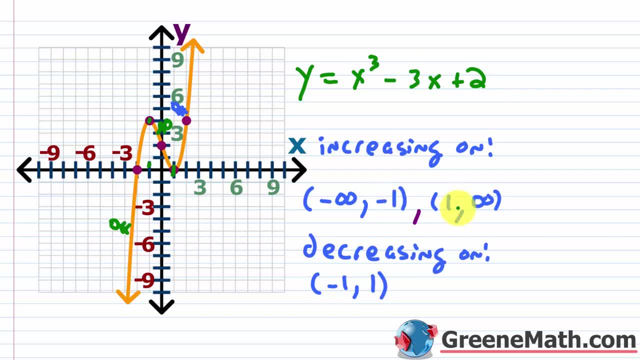 Okay. So if you're given the question in that way, it's okay. But if you're specifically asked for kind of the intervals where the functions increase, where the functions increasing, decreasing or constant, you want to make sure to just kind of use a comma if you have kind of two different intervals there, or use the word. 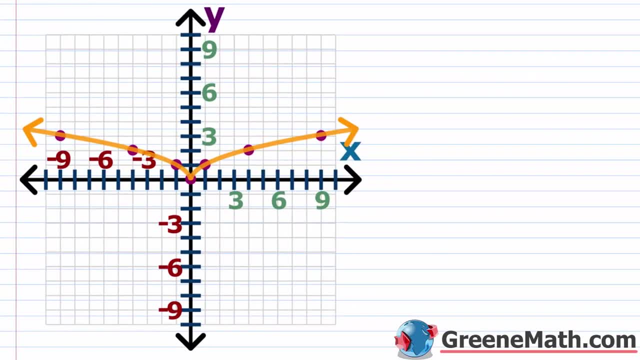 and Okay, And that's all you want to do. All right, Let's look at another. So this guy is going to be. y is equal to the square root of the absolute value of x. So where is it increasing, Where is it decreasing? 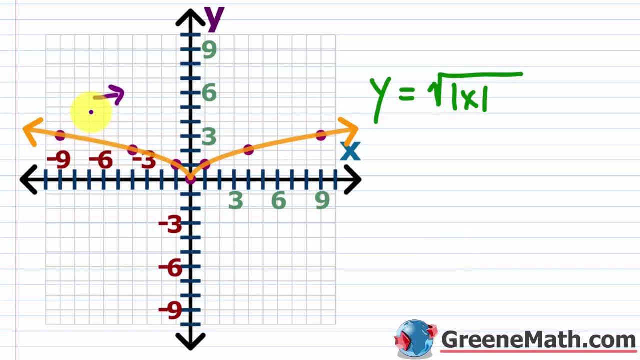 And where is it constant? Well, again, as I move to the right, again, if I draw my stick man figure this guy's going to be walking at a slack. Okay, It's not a slight decline. Okay, It's not a massive decline, but it is decreasing. 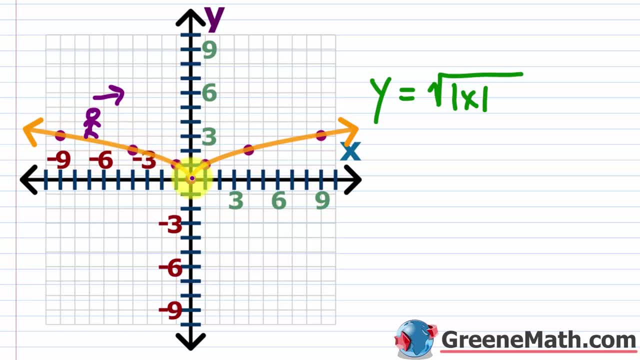 So as I move to the right, it's decreasing from negative infinity up to the point where I get to zero, and then he's going to be increasing out to positive infinity. Okay, So we can say that it's decreasing on the interval from negative infinity to zero again. 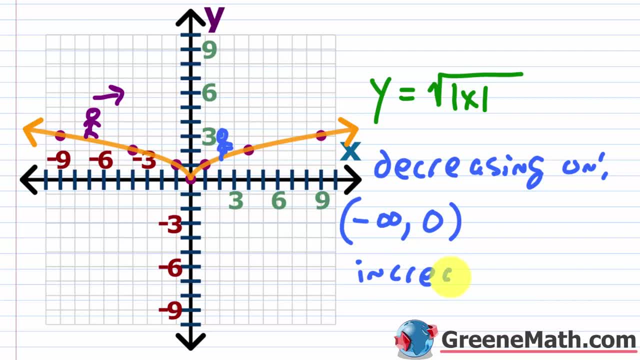 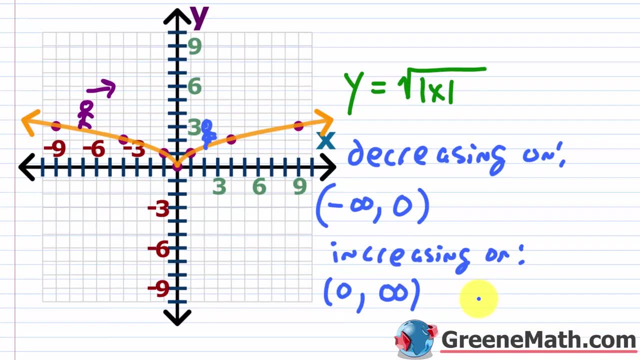 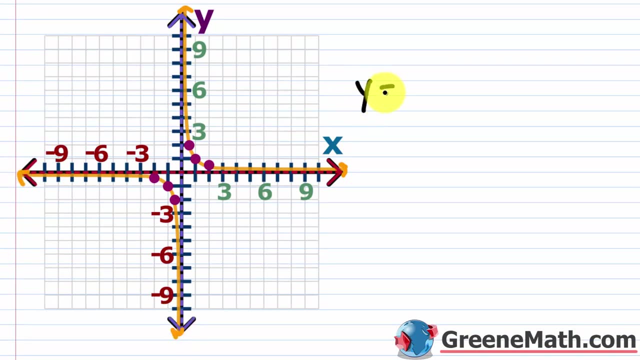 with zero not being included and then increasing, Okay On On the interval from again zero not being included out to positive infinity. What about this guy right here? Let me draw some arrows in here. We should recognize this guy as being the function: y equals one over x. 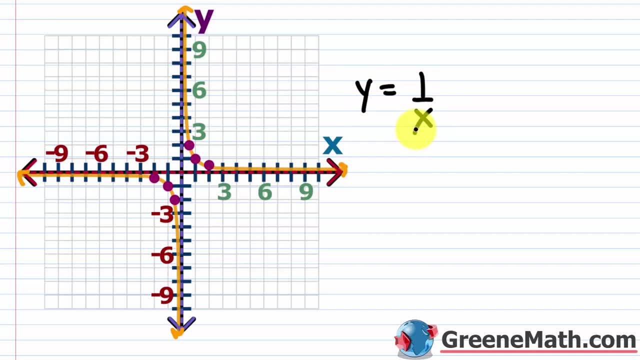 Or again, you could say: f of x equals one over x, if you want. So, essentially, what's happening as I move to the right? Well, from here, remember, we're infinitely close to zero. And as we move to the right, we start decreasing, decreasing, decreasing. 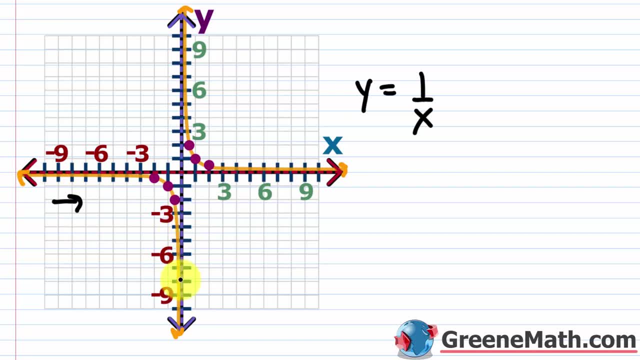 As we approach zero, but we'll never touch it. Okay, So, I know, to kind of the left of zero, I'm always decreasing. Okay, So, from negative infinity to zero, I'm decreasing, So, decreasing on. And from this guy right here, as we move to the right, what's happening? 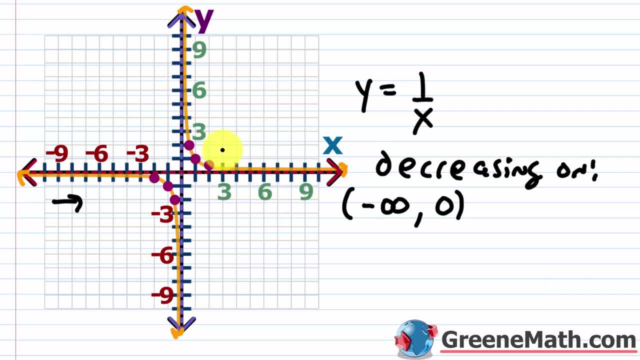 Well, my y values start out up here, basically going to positive infinity. So I'm decreasing And I'm decreasing, And I'm decreasing, I'm decreasing And I'm decreasing infinity, and I'm coming down, down, down, down, down as I move to the right, and I'm still decreasing. 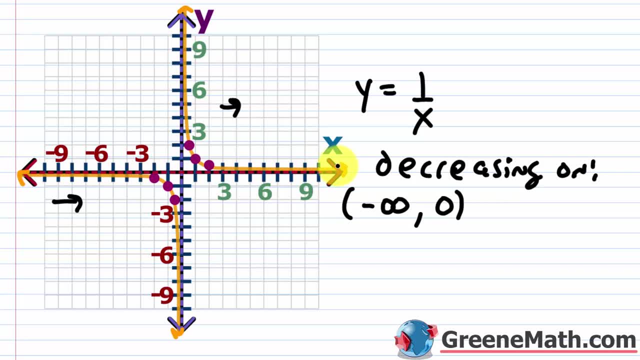 right, I'm going towards a y value of zero, but I'm never going to touch it. I'm going to keep decreasing forever and ever and ever. so I can also say comma again. I'm going to have another kind of thing to list here. we're going to say anything larger than zero out to positive. 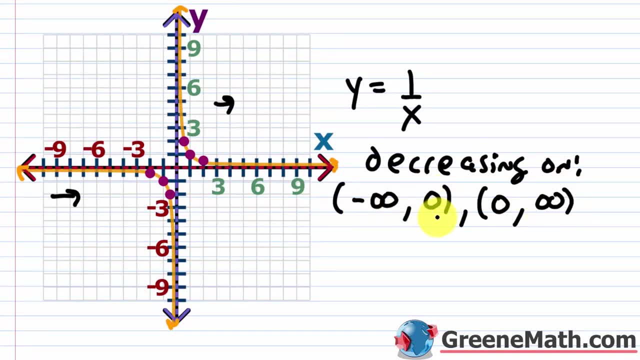 infinity. okay, so from negative infinity to zero- not included- and then from zero to infinity, again zero, not included. again, don't put a union symbol in there. that's not correct. all right, for the final example, I'm going to give you one that's just kind of made up. this is a drawing that I 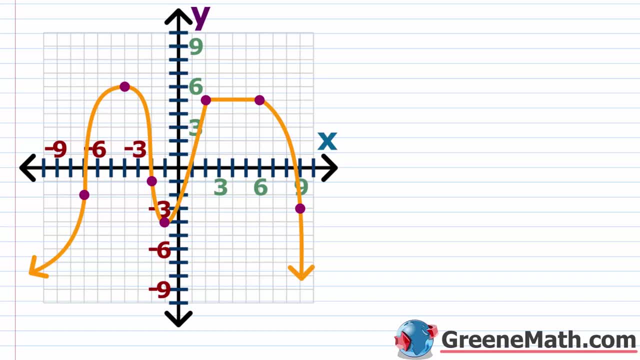 came up with. you'll see a lot of these in your textbook. just to give you a couple of examples where you have some kind of constants, some decreasing, some increasing, a lot of stuff going on. so if we look at this guy again, if I use my little stick figure, what's going on here is that. 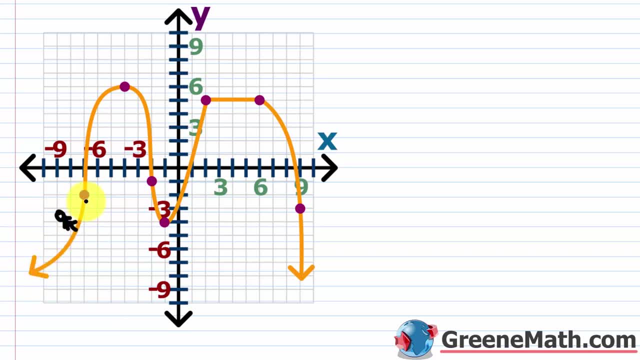 we start out as we come from negative infinity, we're going to be increasing up to the point where we're going to be decreasing, up to the point where we're going to be increasing up to the point where we're going to be increasing up to the point where we're going to be increasing up to the. 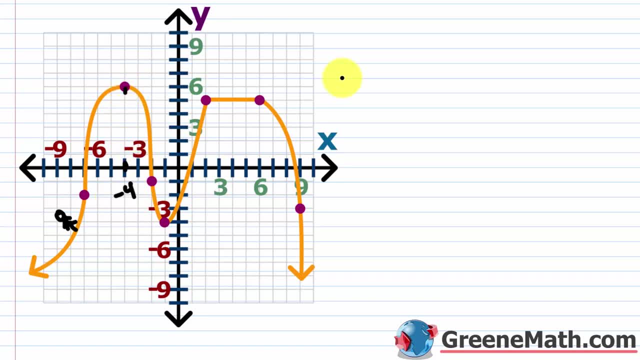 point where we get to an x value of negative four. okay, so let me just write this: we're going to say increasing on, so from negative infinity up to not including negative four, and then let me put decreasing on, so, decreasing on, so next the stick figure is going to be walking downhill. 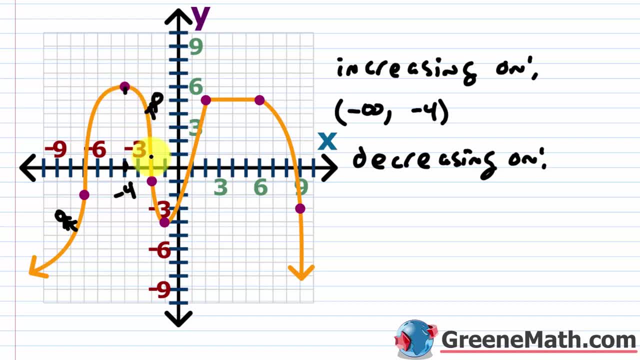 right, starting at negative four, that x value going all the way up to an x value, that is negative one. okay, this is negative one here. so we'll say from negative four to negative one again. neither of those is going to be included. let me make this a little better. so negative four. 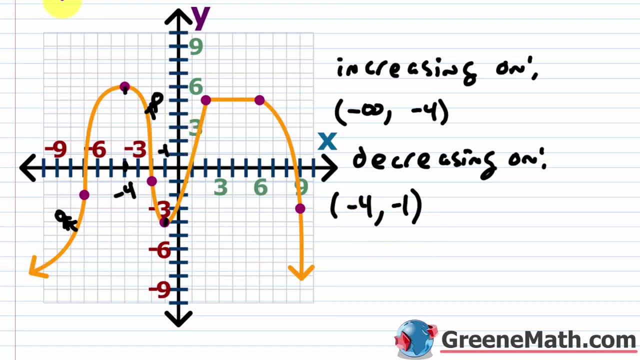 negative one. and then this guy right here again- let me kind of change colors- he's going to start walking uphill now, starting at an x value of negative one. he's walking uphill until he gets to an x value of two. okay, so it's going to be increasing. the other interval is going to be: